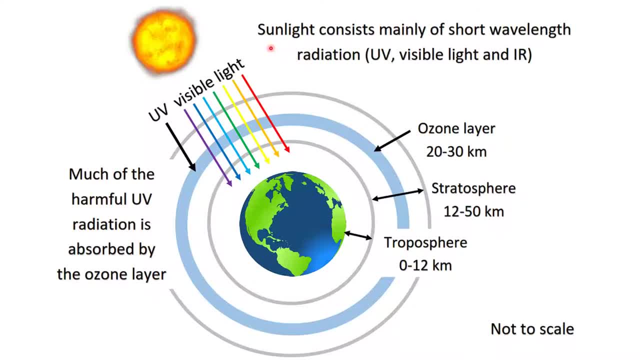 Sunlight consists mainly of short wavelength radiation, that's mainly UV, visible light and infrared. As we can see, visible light is able to pass through the ozone layer. Much of the harmful UV radiation from the sun is absorbed by the ozone layer. So next we look at how this harmful UV 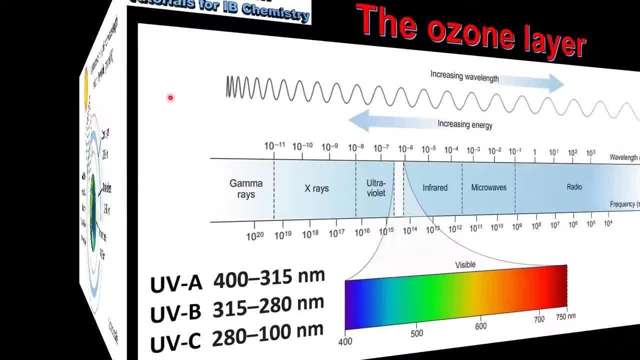 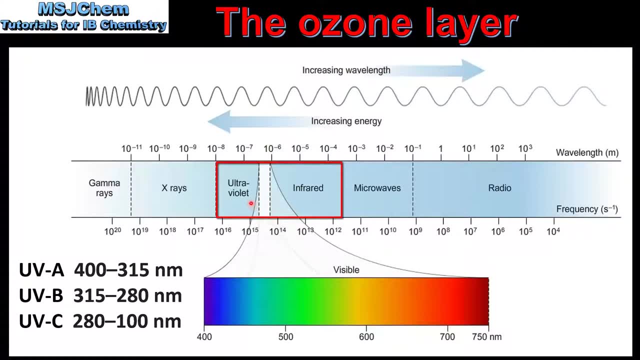 radiation is absorbed in more detail, So we'll start by looking at the electromagnetic spectrum. Here we can see the infrared, visible light and ultraviolet regions, As we saw in the previous. from these three regions, However, the ozone layer is responsible for absorbing harmful UV radiation. 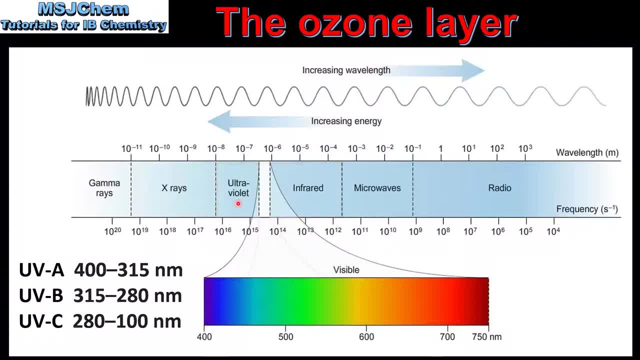 So for the rest of the video we'll focus on this region. Ultraviolet radiation can be divided into UVA, UVB and UVC. UVA has the longest wavelength and UVC has the shortest wavelength. In terms of UVC, UVA has the longest wavelength and UVC is the highest energy UV radiation, As we'll see in the 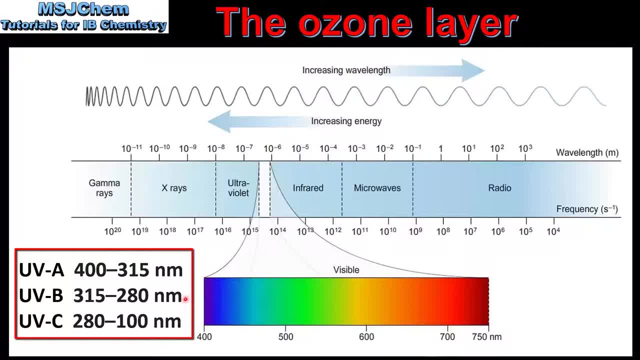 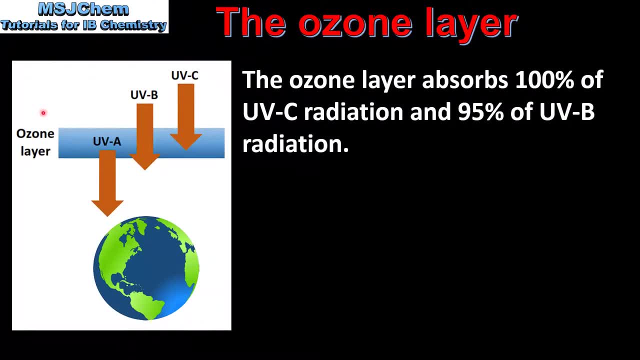 next slide, the ozone layer mainly absorbs UVB and UVC radiation. So, as we saw in a previous slide, UV radiation can be divided into UVA, UVB and UVC. As we can see from this diagram, the ozone layer absorbs 100% of UVC radiation and approximately 95% of UVB. 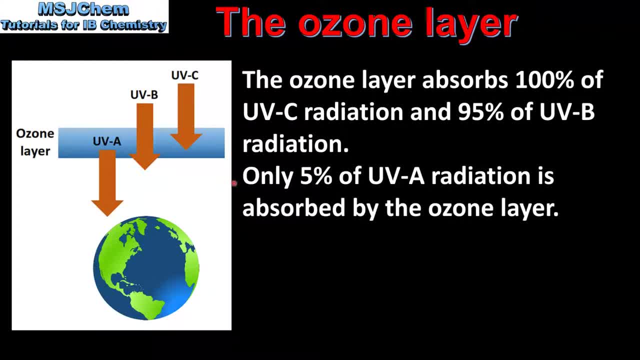 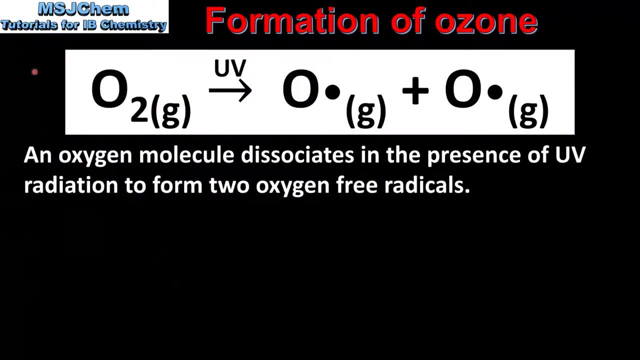 Only 5% of UVA radiation is absorbed by the ozone layer. Both UVA and UVB can damage the DNA in skin cells, which can cause skin cancer and premature aging. Next we look at the formation and destruction of ozone, So starting with the formation in the first step, an oxygen molecule. 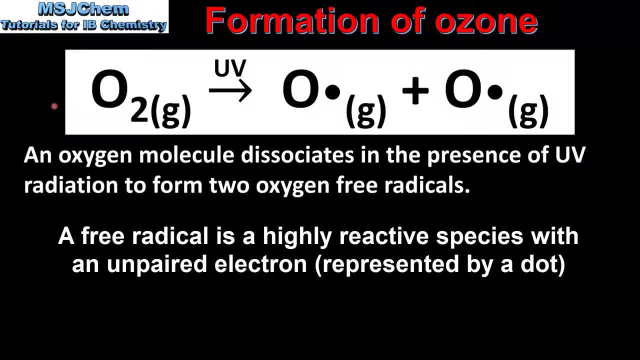 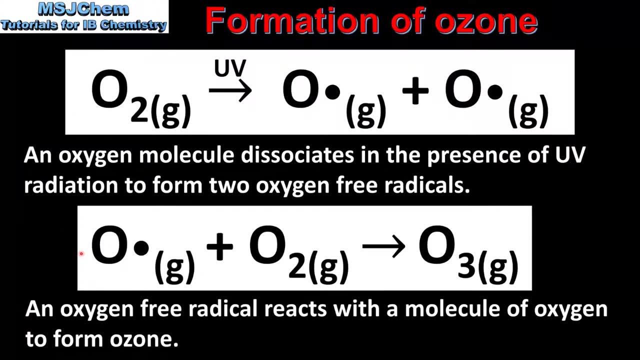 dissociates in the presence of UV radiation to form two oxygen-free radicals. So in this equation we have our oxygen molecule, which dissociates to form two oxygen-free radicals. In the next step, an oxygen-free radical reacts with a molecule of oxygen to form ozone. So 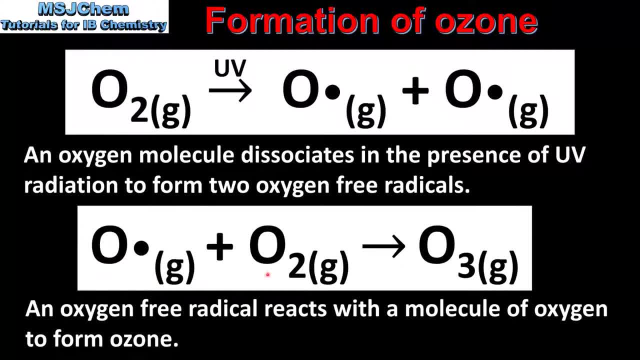 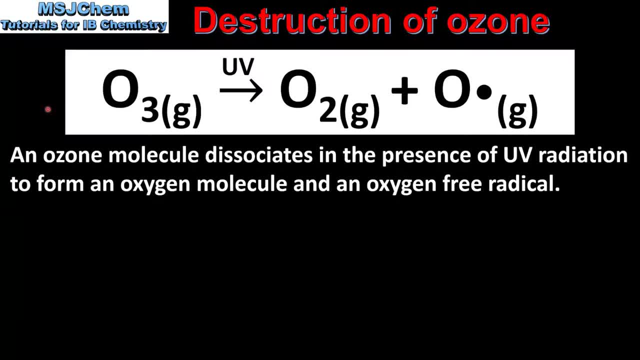 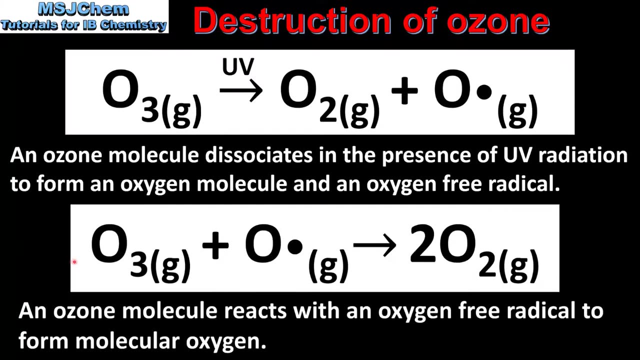 here we can see our oxygen-free radical reacting with an oxygen molecule to form a molecule of ozone. Next we look at the destruction of ozone. Ozone can be broken down in two ways. In this reaction, an ozone molecule dissociates to form a molecule of oxygen and an oxygen-free radical. The second way in which ozone can. 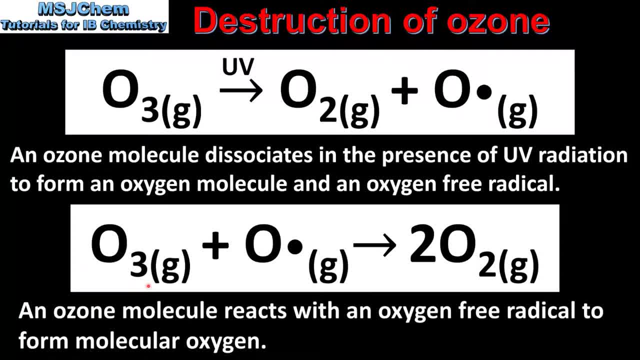 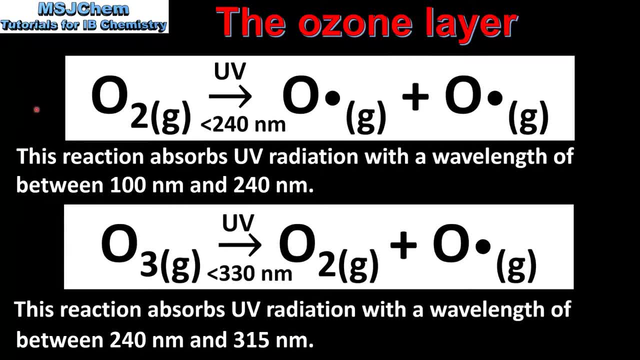 be broken down is when an ozone molecule reacts with an oxygen-free radical to form two molecules of oxygen. So we'll finish the video by looking at the significance of the UV radiation absorbed in these two reactions. The first reaction, which is the first step in the formation of 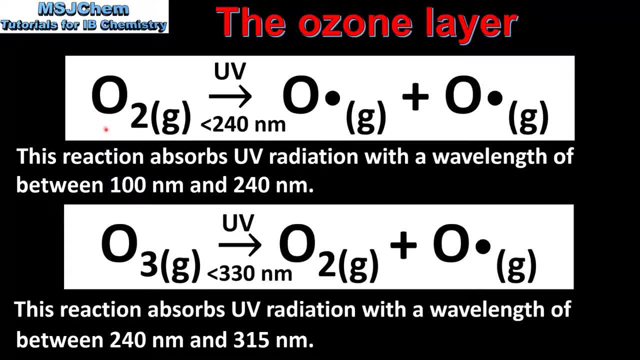 ozone absorbs UVA. The second reaction, which is the first step in the formation of ozone, absorbs UV radiation with a wavelength of between 100 and 240 nanometers. The second reaction, in which ozone dissociates to form oxygen and an oxygen-free radical. 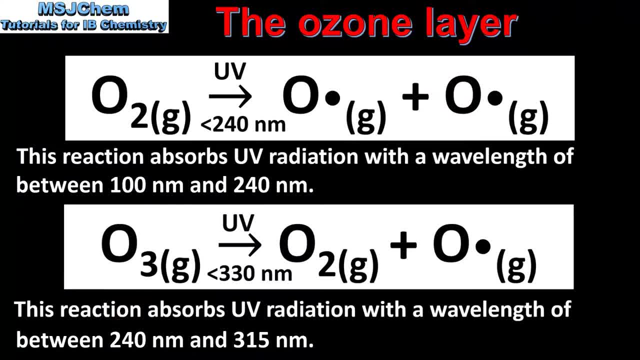 absorbs UV radiation with a wavelength of between 240 and 350 nanometers. So, to summarize the wavelengths of UV radiation absorbed in these two reactions correspond to UVB and UVC radiation. So, to summarize, the wavelengths of UV radiation absorbed in these two reactions correspond to UVB and UVC radiation. 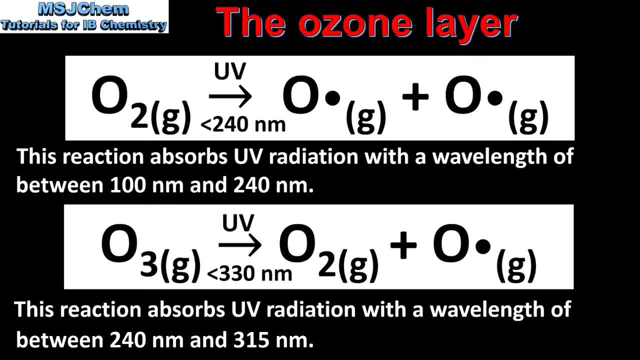 So to summarize, the wavelengths of UV radiation absorbed in these two reactions correspond to UVB and UVC radiation. So from this we can see that the formation and destruction of ozone absorbs harmful UV radiation. So that's all from this video. in the next video we'll be looking at the bonding in oxygen. and ozone in more detail. 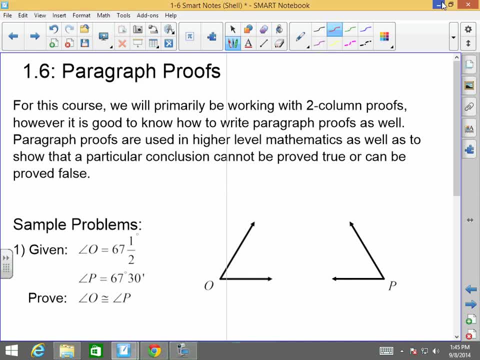 Good morning, afternoon or evening, How y'all doing today. Welcome back to Mr Morrow's Geometry class. Today we're going to be talking about paragraph proofs, okay, And for this course we will primarily be working with two-column proofs, which we have already seen.